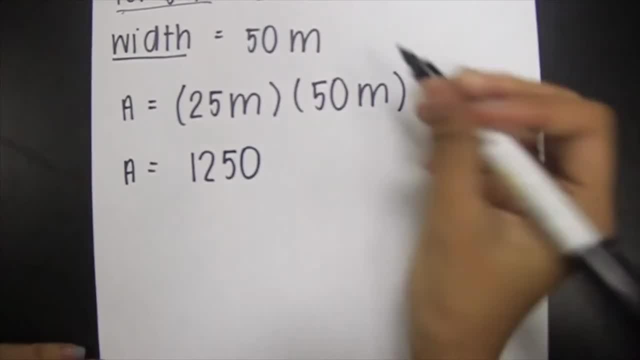 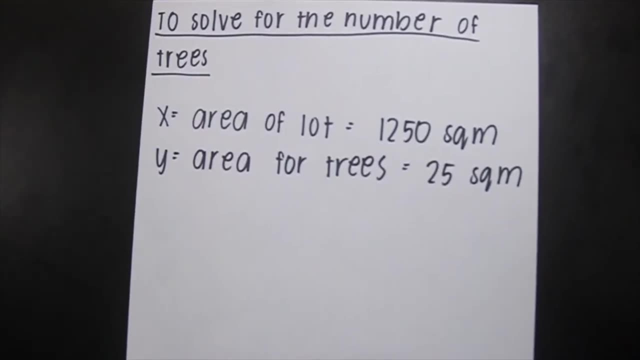 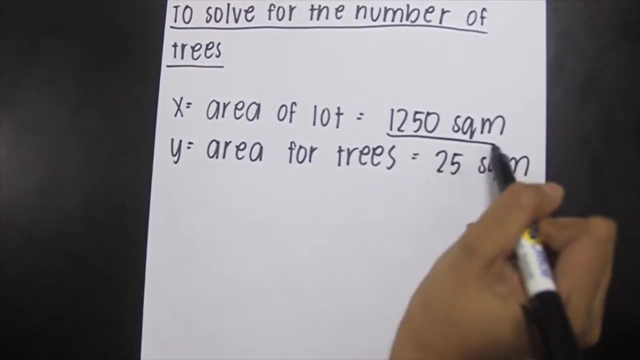 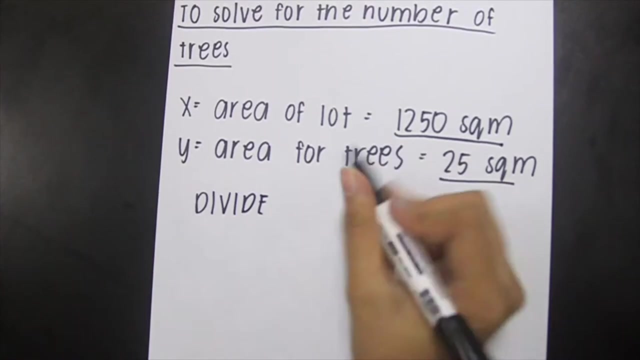 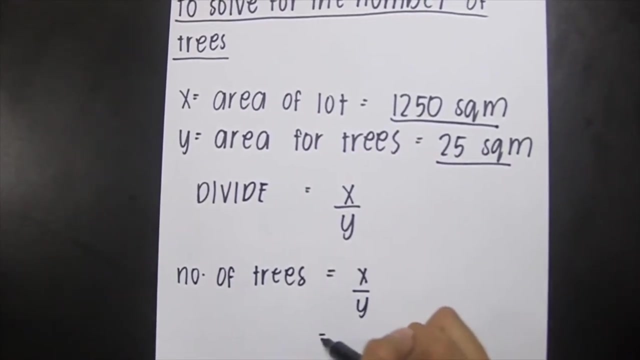 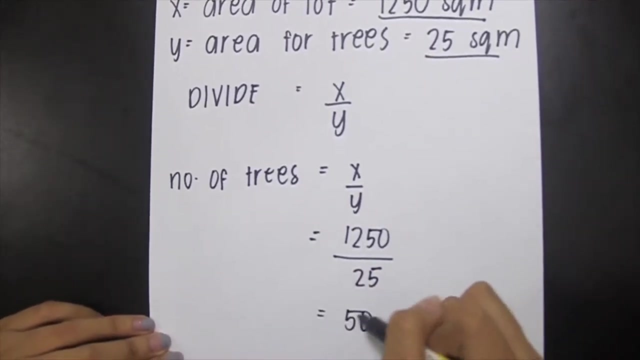 equal to one thousand two hundred fifty square meters. To solve for the number of trees that will be planted, use the values of the area of the lot and the area allotted for each tree. Divide the values, The number of trees equals to one thousand two hundred fifty over twenty five equals to fifty. 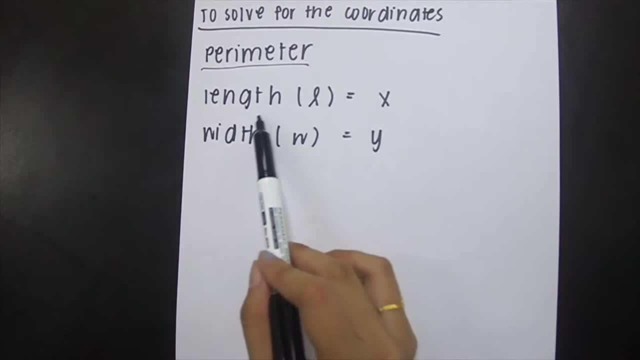 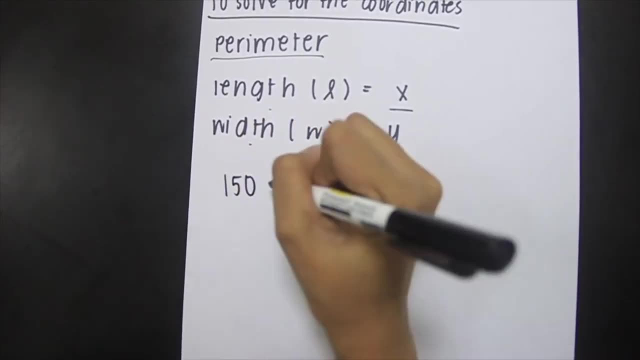 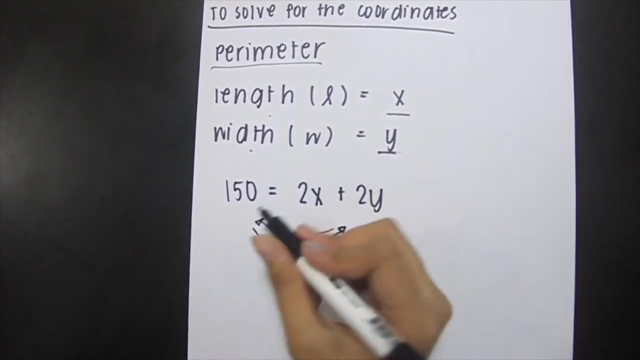 To solve for the coordinates of this nonlinear equation, use the formula for finding the perimeter. Let the length be x and the width be y. One fifty is equal to two x plus two y Through symmetric property of equality. let's make two x plus two y be equal to one hundred fifty. 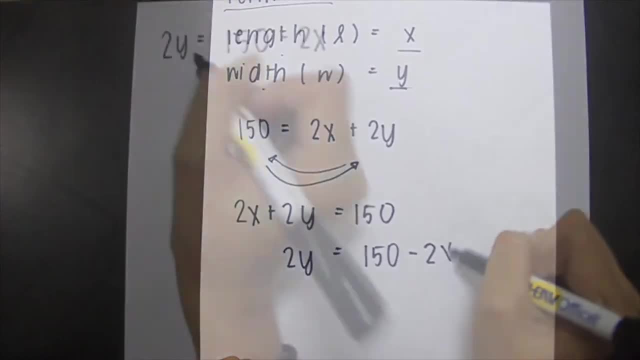 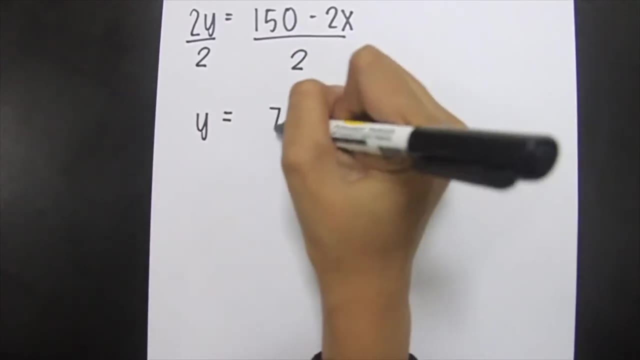 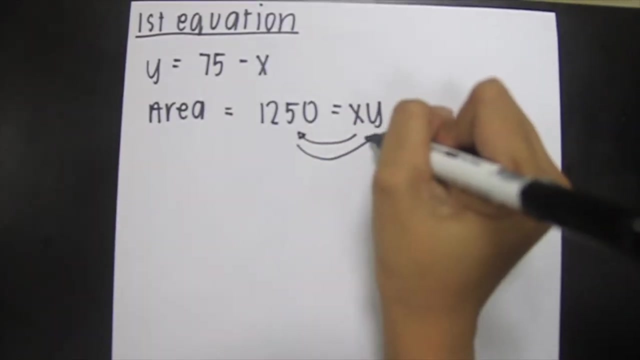 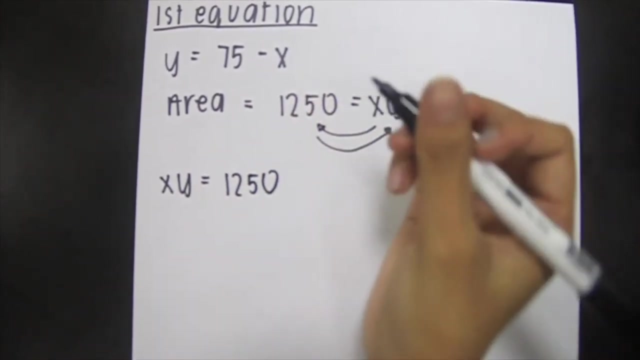 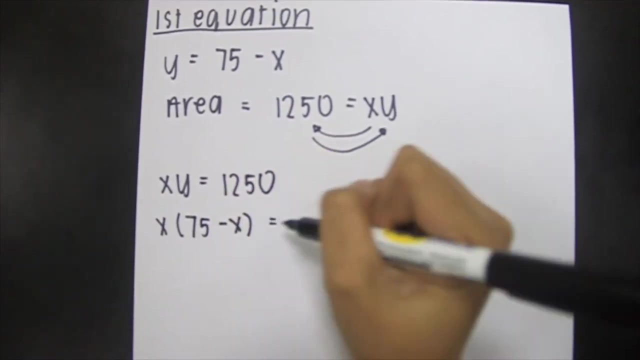 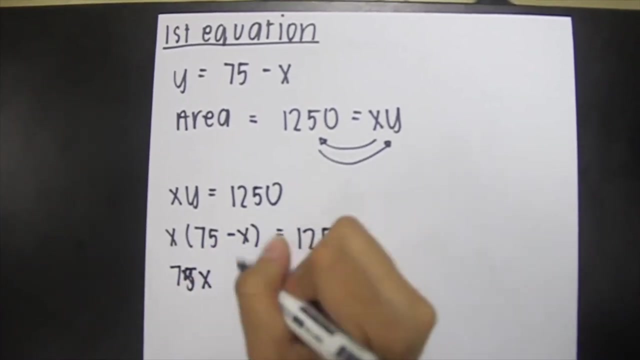 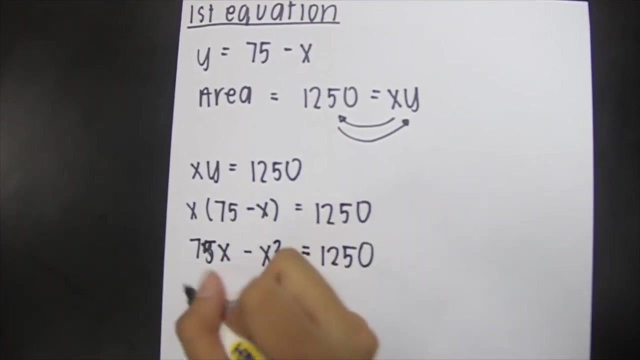 Transpose two x, Divide both sides by two to come up with: y is equal to seventy five minus x. To solve for x use the formula: y is equal to one thousand two hundred fifty. Substitute the y value, Distribute x, Interchange, so negative x squared is the first term. 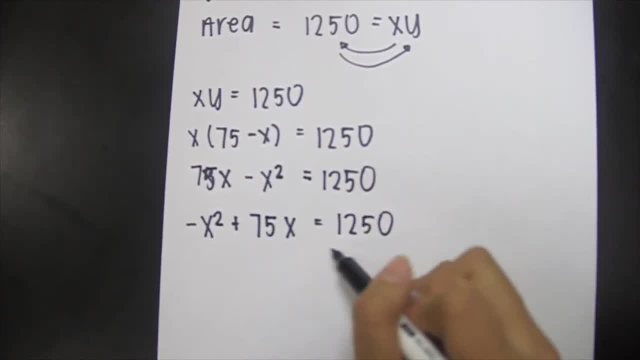 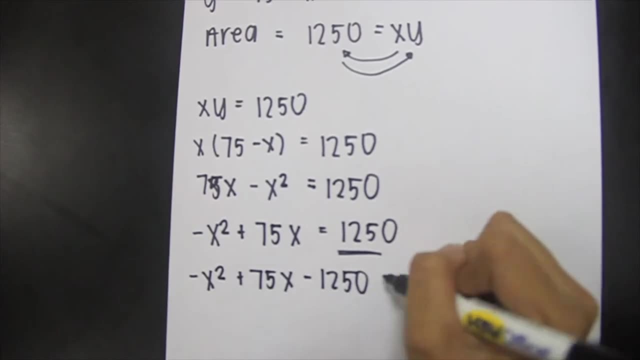 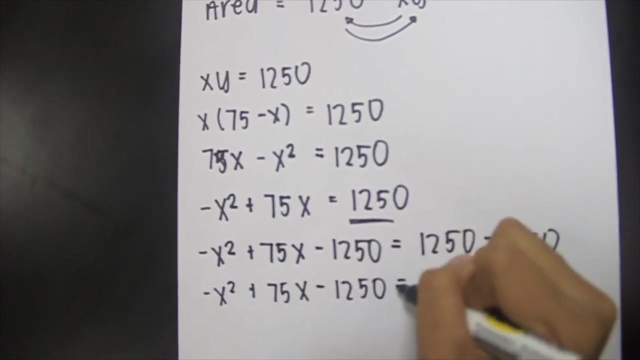 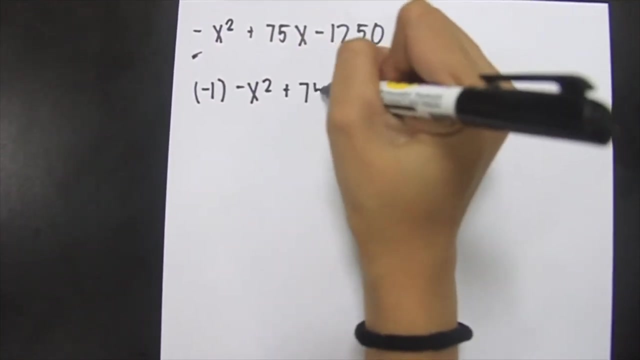 Make the right side of the equation be equal to zero. Multiply negative one to make x positive. Add x to positive. 1. Add x to negative. 1. Add x to positive. 1. Add x to negative. 2. Make the right side of the equation be equal to zero.